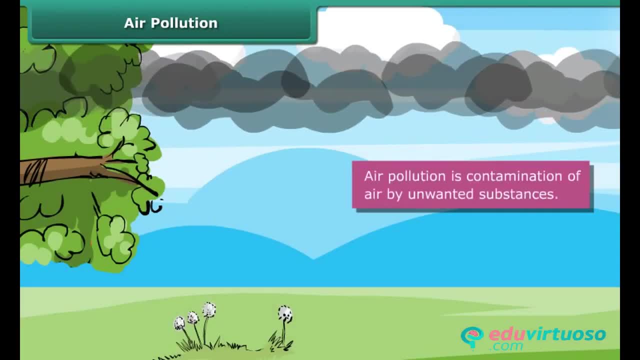 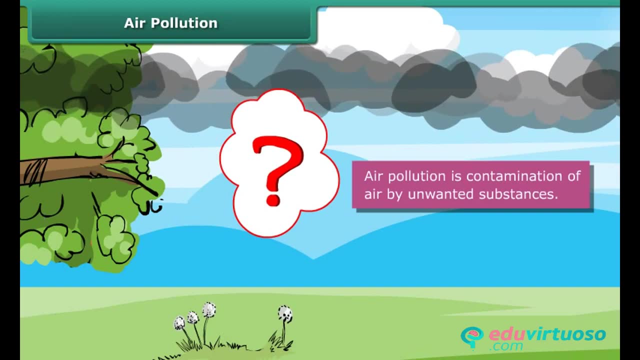 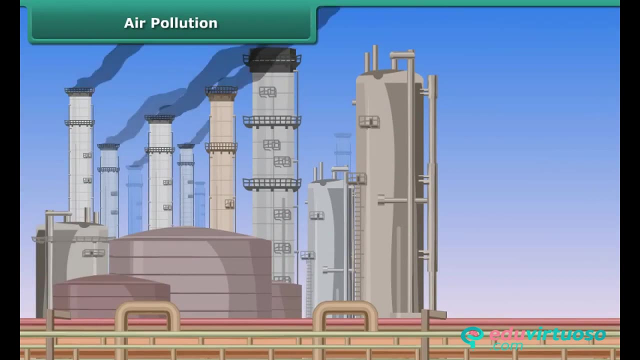 But air is getting polluted day by day due to presence of unwanted substances in it. Now you would like to know from where these substances come. These are released when fuels burn in vehicles. Factories and power plants produce them as gaseous wastes. 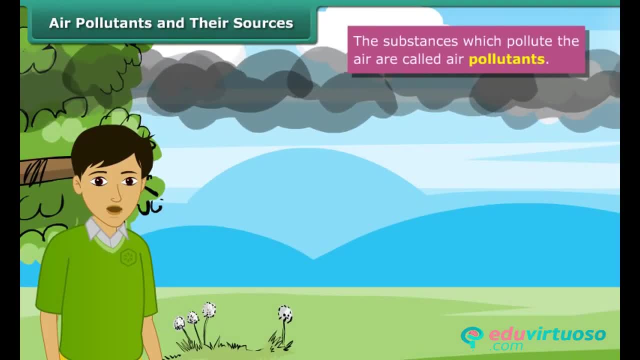 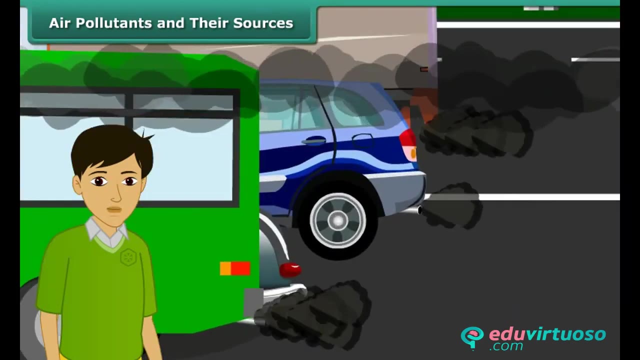 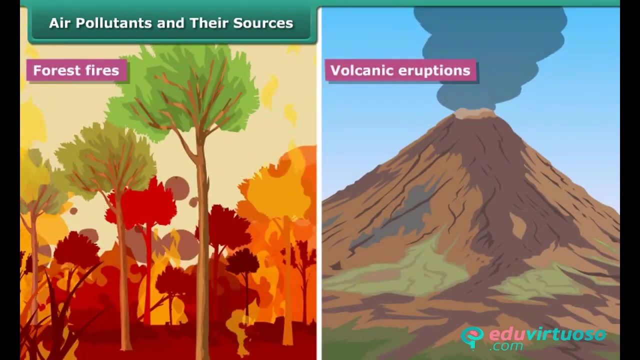 Which substances pollute air? The toxic gases like carbon dioxide, sulfur dioxide, nitrogen dioxide and carbon monoxide. These are often released by the engines of vehicles, Like the engine of a car, Like trucks and buses. Sometimes they may come from natural sources, like smoke and dust arising from forest fires or volcanic eruptions. 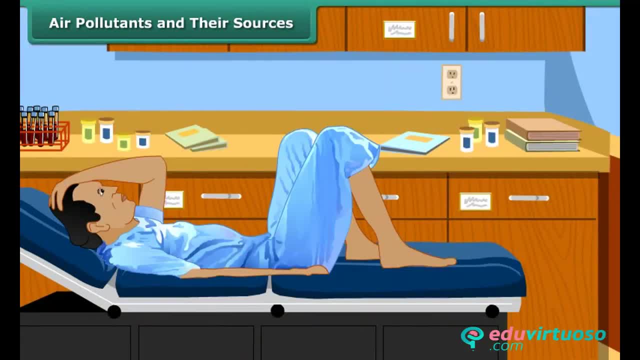 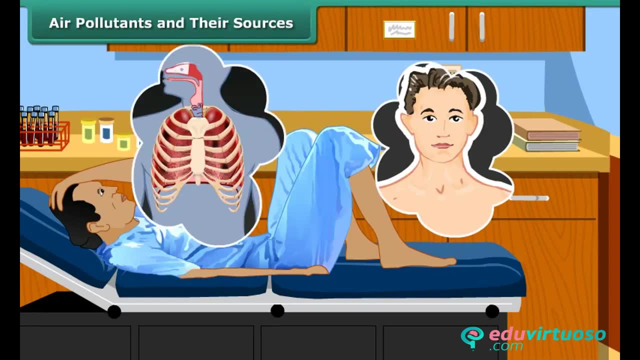 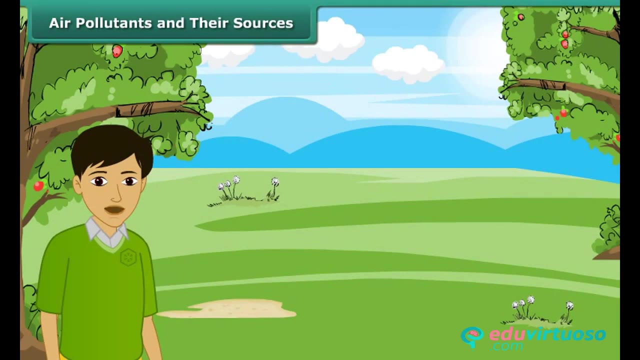 These gases can make healthy people sick and sick people even worse. They affect your eyes and throat. In some cases, they can permanently damage your lungs and even cause cancer. Have you heard of smog? Smog is made up of smoke, Smoke and fog. 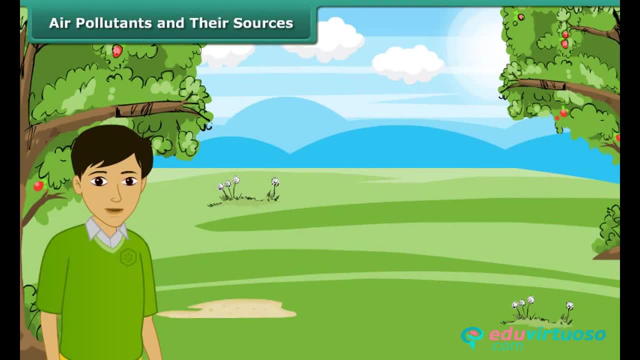 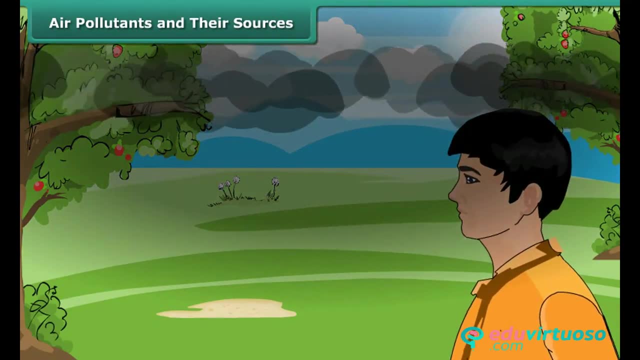 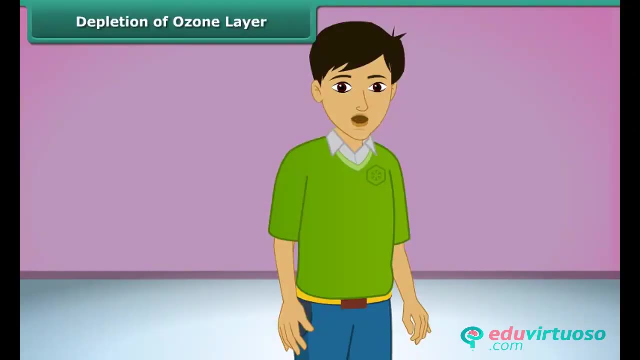 Smoke generally contains oxides of nitrogen and other air pollutants. The smog causes breathing difficulties such as asthma, cough and wheezing in children. Let us learn about ozone layer. It is a layer of ozone gas in the upper atmosphere of earth. 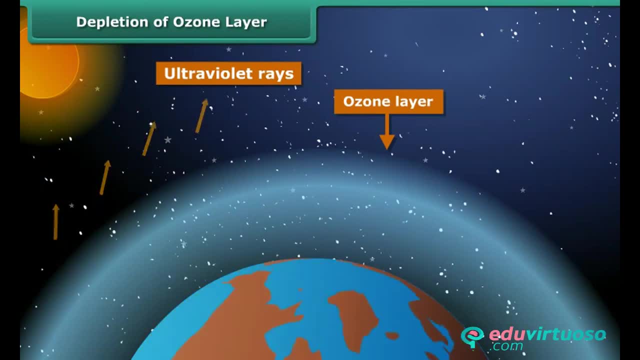 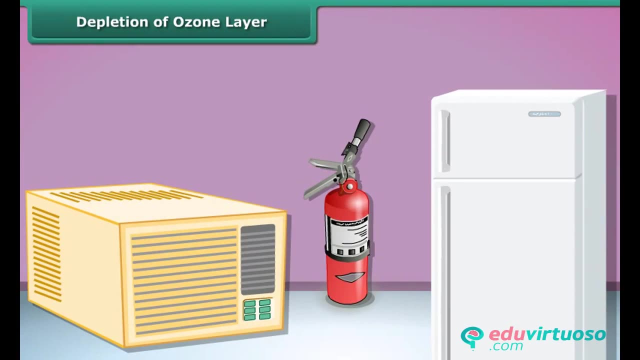 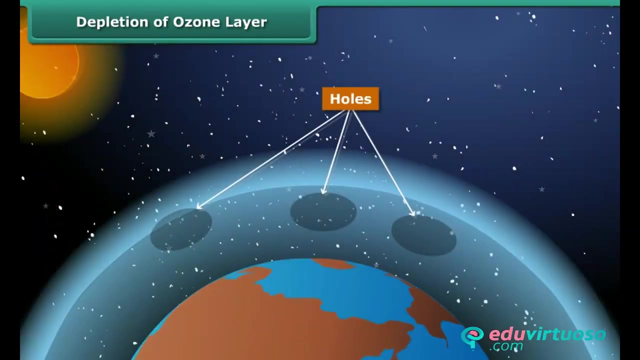 What is its role? It protects us from harmful ultraviolet rays of the sun. Things like air conditioner, refrigerators and fire extinguishers release chlorofluorocarbons into the atmosphere and create holes in the ozone layer. CFCs are another type of air pollutants. 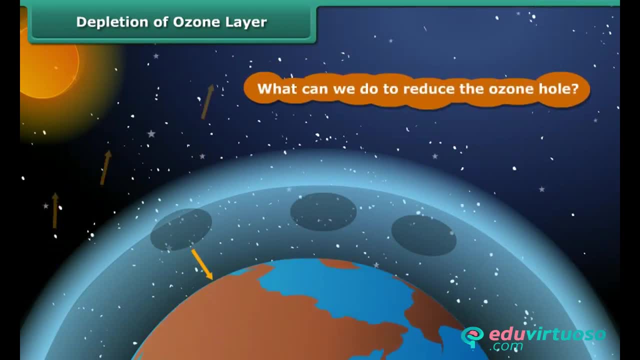 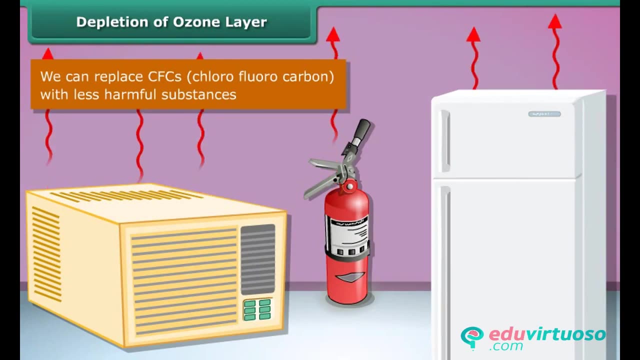 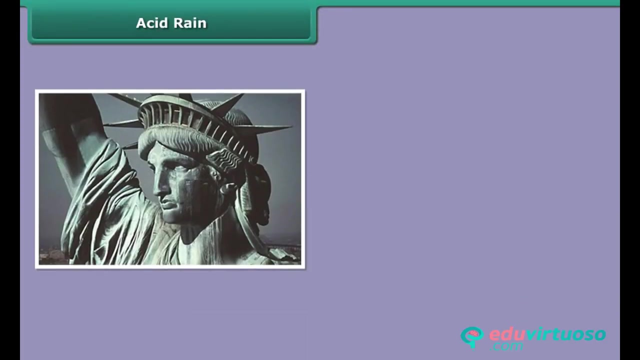 What can we do to reduce the ozone hole? We can replace CFCs with less harmful substances to save the ozone layer from depletion. Students, this is a simple interactivity for you. These are the images of Statue of Liberty in New York and Taj Mahal in Agra. 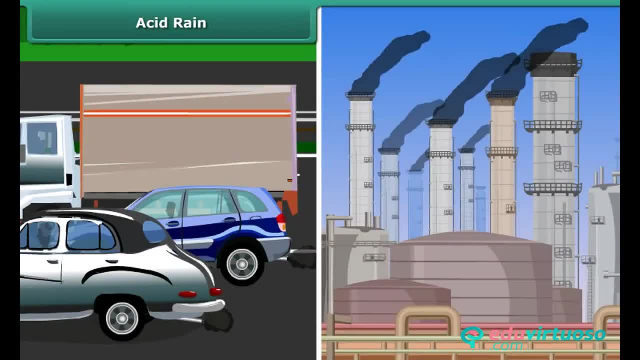 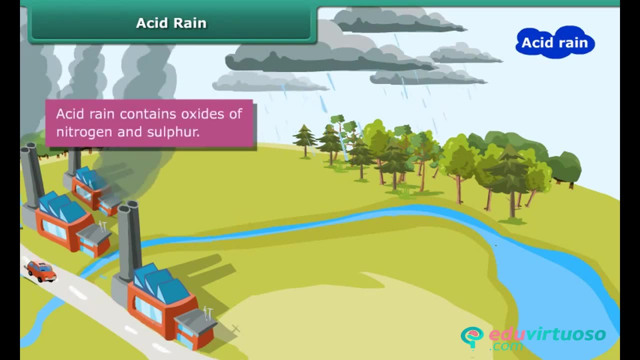 They are badly damaged due to acid rain. Do you know what causes acid rain? Industries and vehicles release toxic gases like sulfur dioxide and nitric oxide into the atmosphere. These gases react with the water vapors present in the atmosphere to form sulfuric acid and nitric oxide. 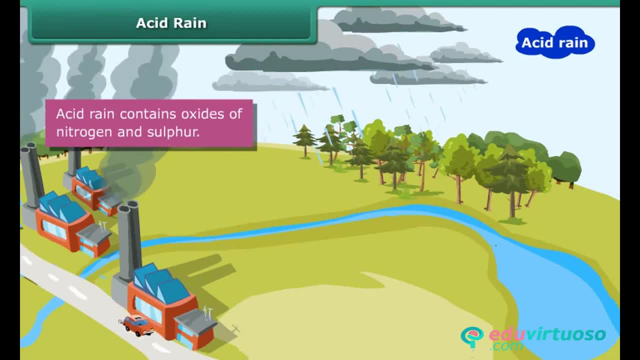 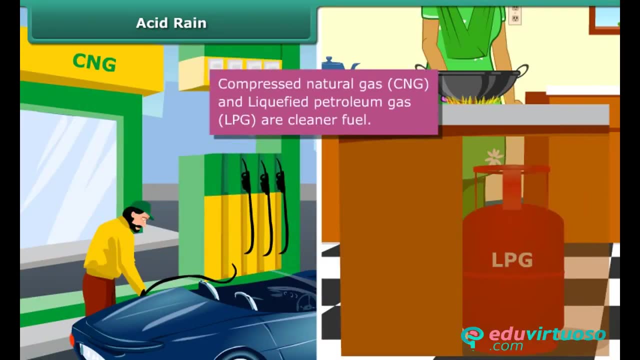 Which fall as acid rain. What can reduce the acidic rain? Use of clean fuels like compressed natural gas and liquefied petroleum gas can reduce the acidity of rain. It's freezing. This may ruin the plants. You know, there is a way to save these plants from this extreme cold. 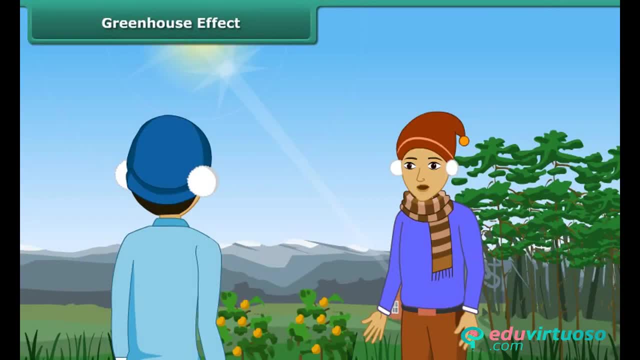 It's freezing. This may ruin the plants. You know there is a way to save these plants from this extreme cold. It's freezing, It's freezing. You know there is a way to save these plants from this extreme cold. What is that? 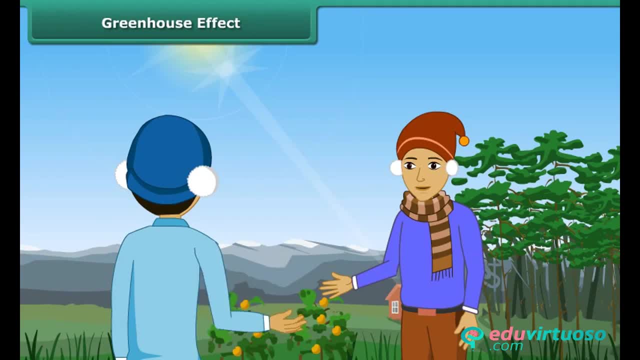 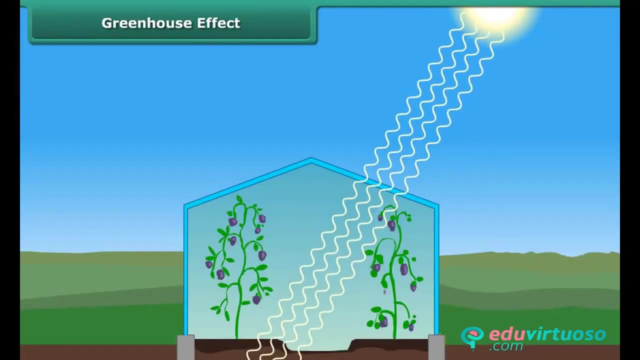 We can use greenhouse effect to protect them from cold. What is greenhouse effect? See this house. This has so many glass panes. This is called greenhouse. When solar rays come into this house, heat up the air inside it. That hot air is trapped inside. 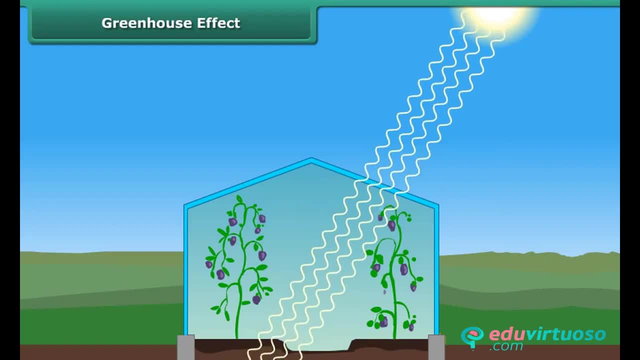 which makes nice, warm and humid environment for plants to grow, which makes nice, warm and humid environment for plants to grow. Similarly, the greenhouse gases like carbon dioxide, methane and nitric oxide in the atmosphere act like glass panes When the sun's radiation reaches. 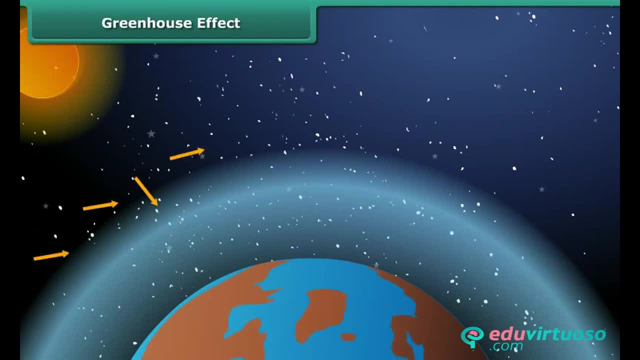 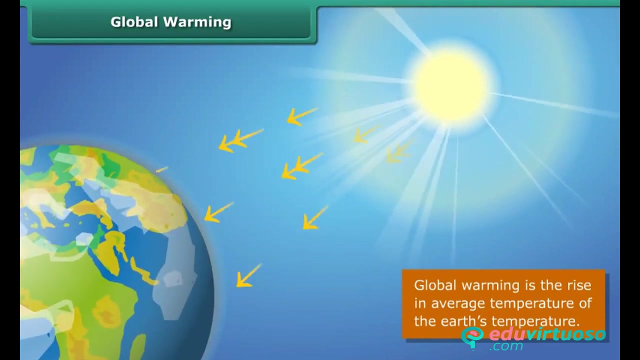 our atmosphere. some rays are reflected back into space. some rays are reflected back into space and some are trapped into greenhouse gases, causing the atmosphere of the earth to warm up. to warm up, global warming means earth is heating up. scientists believe that earth's temperature is going. 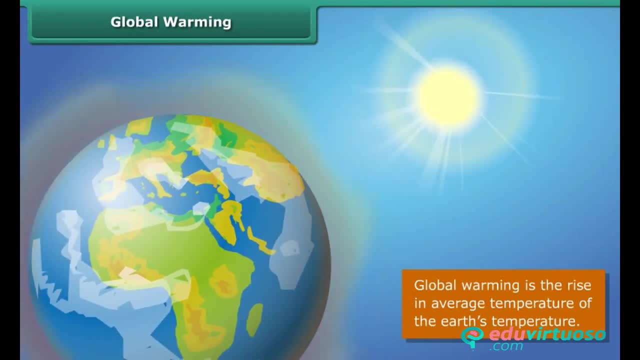 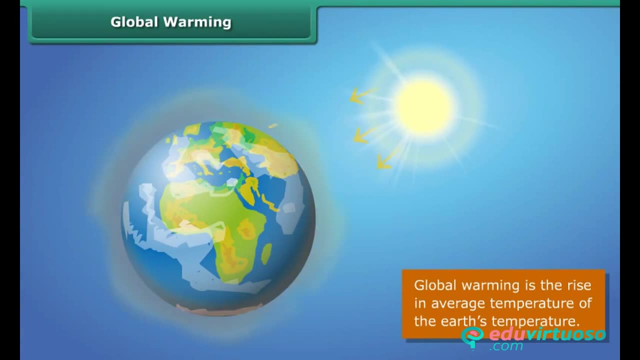 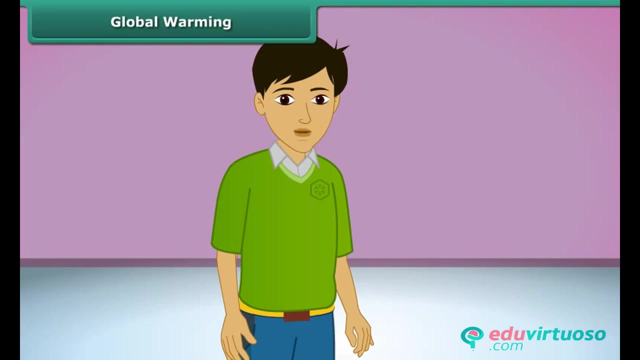 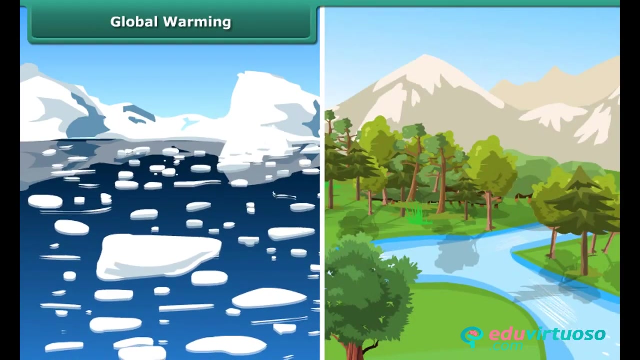 to increase even more in coming years. scientists say that the greenhouse gases, like carbon dioxide, trap the heat from sun and increase the temperature of earth's atmosphere. can you imagine the consequences of heating of earth's atmosphere? it will melt the ice at poles, causing the sea levels to rise, which could flood the low-lying areas, thus affecting 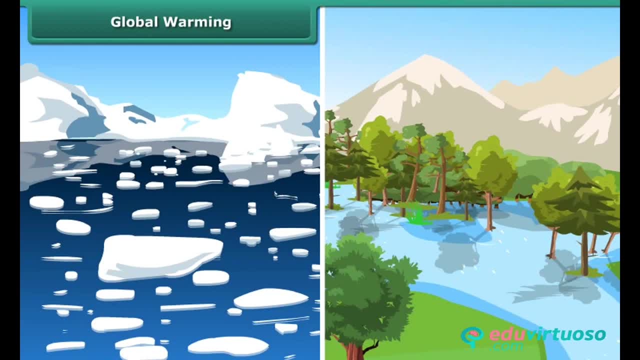 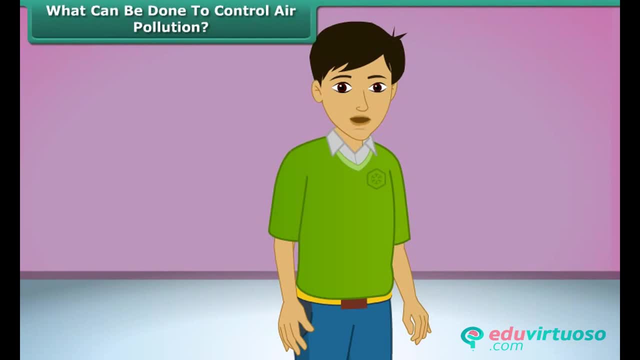 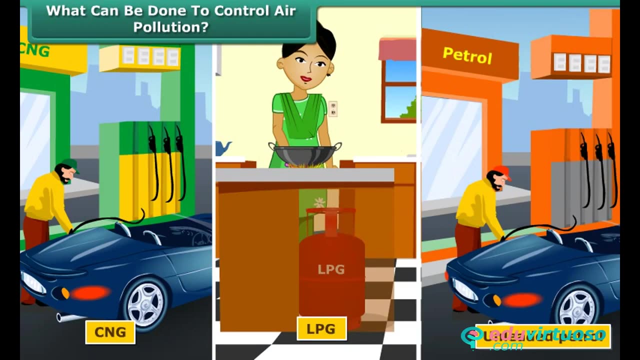 the habitats of plants, animals and people. students, can you tell what should we do to reduce air pollution? there are many things we can do. we can use clean fuels such as cng, lpg and unleaded petrol instead of fossil fuels. we can use solar energy, hydro power.